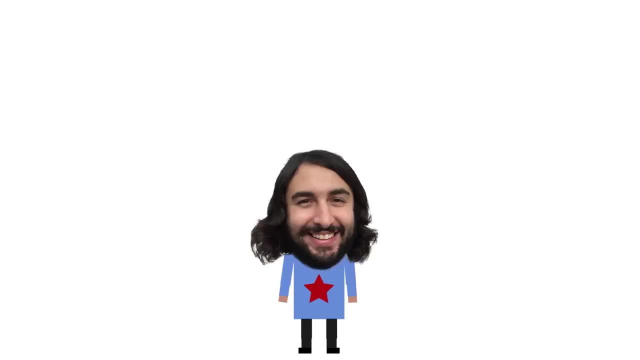 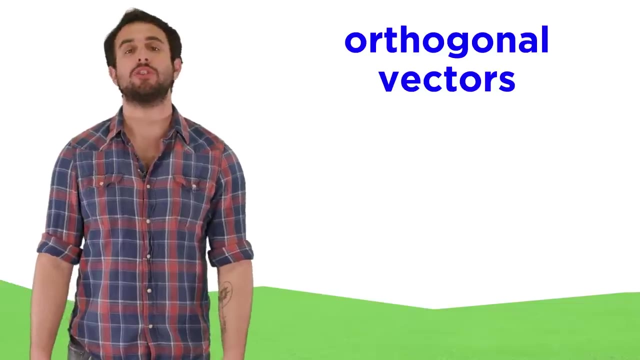 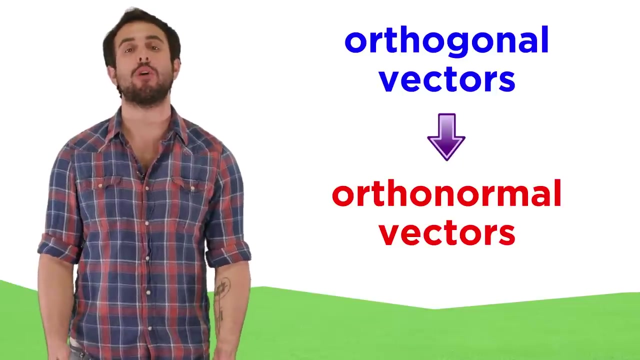 Professor Dave, here I want to teach you the Gram-Schmidt process. In the previous tutorial we learned all about orthogonal vectors and how we can generate from these a set of orthonormal vectors by taking each vector and dividing it by its. 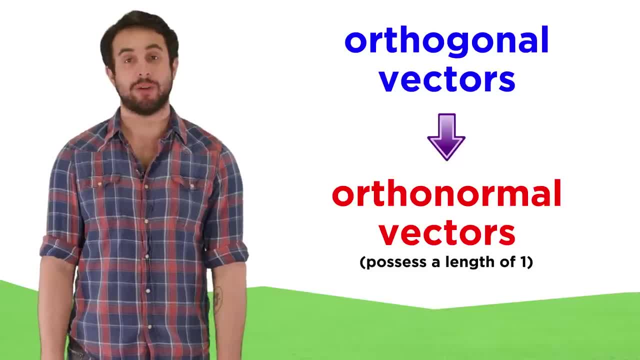 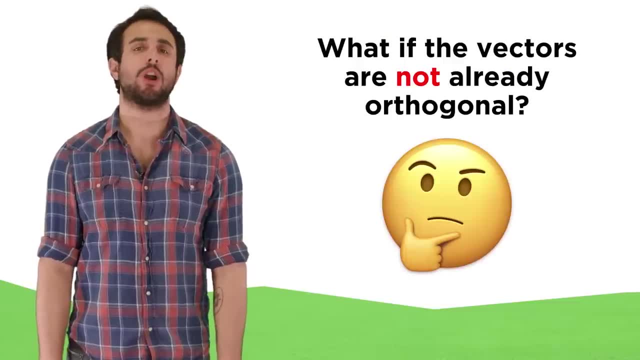 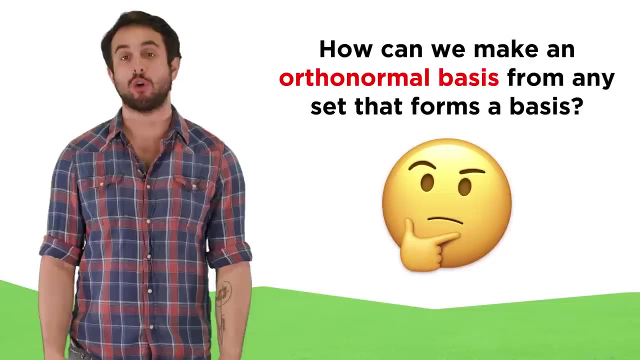 length. This makes each vector's length equal to one and, since they were already orthogonal, the new vectors become orthonormal. But what if we start with a set of vectors that are not already orthogonal? Furthermore, how do we go about making an orthonormal basis for a vector space given? 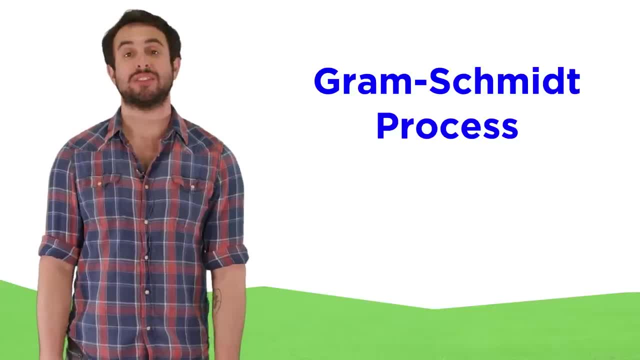 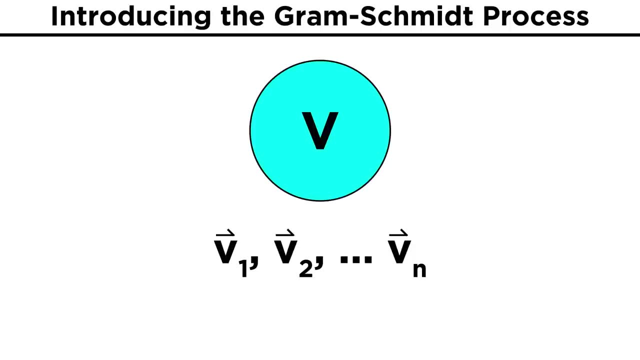 any set of vectors that form a basis To do this, we need to learn something called the Gram-Schmidt process. so let's take a look at this now To see how this works. let's examine the vectors V1 to Vn, which serve as the basis. 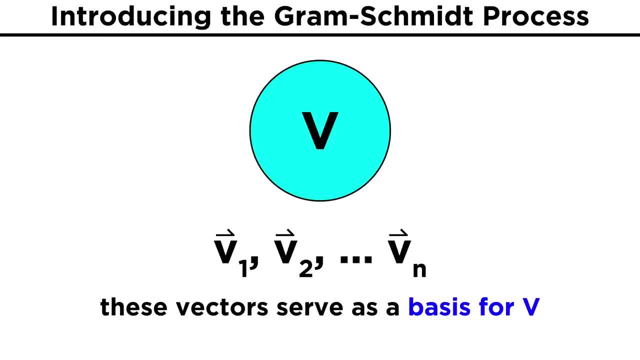 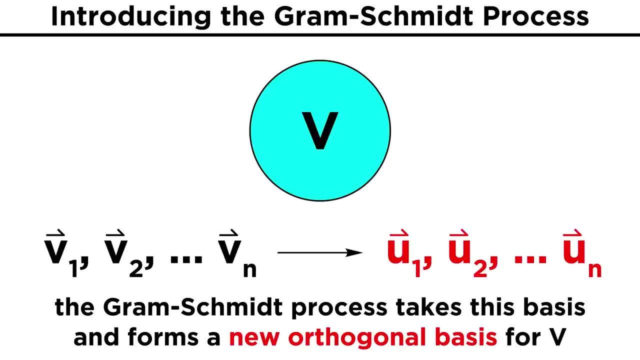 for the vector space V. Our only requirement for these vectors is that they form a basis. We are no longer assuming any orthogonality between them. The Gram-Schmidt process takes these vectors and forms a new orthogonal set of basis vectors. 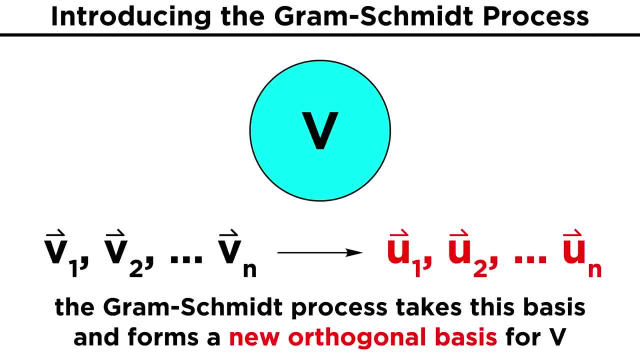 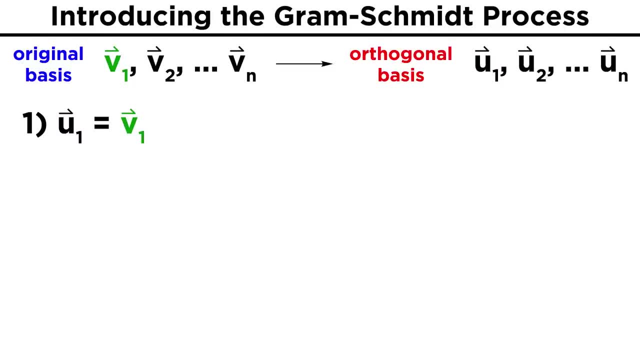 which we will label U1 to Un. The process goes as follows: First, start by setting the first new vector U1, equal to the first vector U1. For the second step, take the second vector, V2, and subtract from it the inner product. 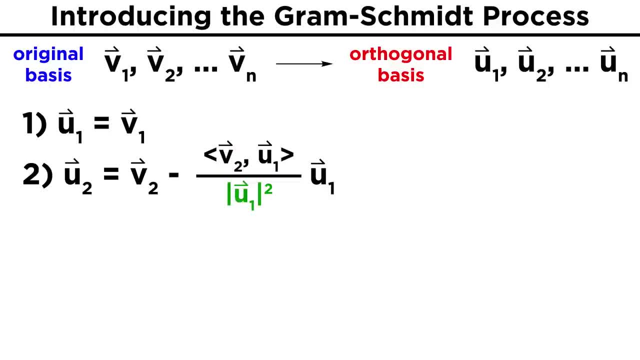 between V2 and U1, divided by the length of U1, squared times the vector U1.. So all together that looks like this. Then the third step will be to take the vector V3, and subtract a similar term. The only difference is that now we take the inner product between V3 and U1, and subtract. 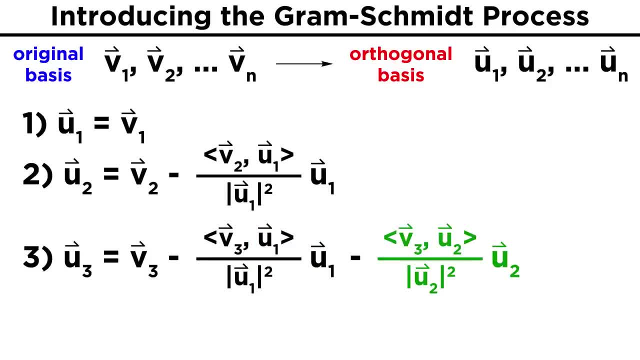 a similar term. The only difference is that now we take the inner product between V3 and U1. And then we also subtract another term, which is the inner product between V3 and U2, divided by the length of U2, squared times U2.. 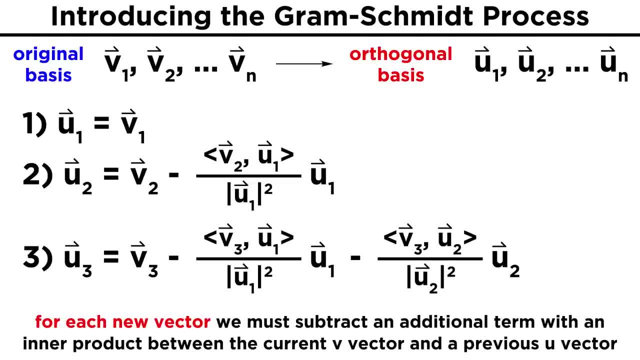 At this point, you may notice a pattern emerging: For each new vector, we must subtract an additional term that involves the inner product of the current V vector with each previously found U vector, so we will need one more such term for each vector. The reason we need to do this is that we are subtracting off any part of the V vector. 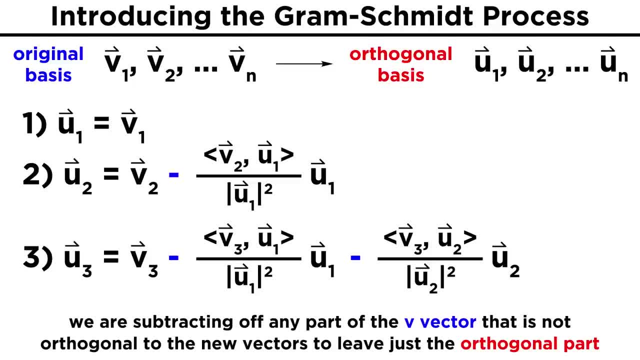 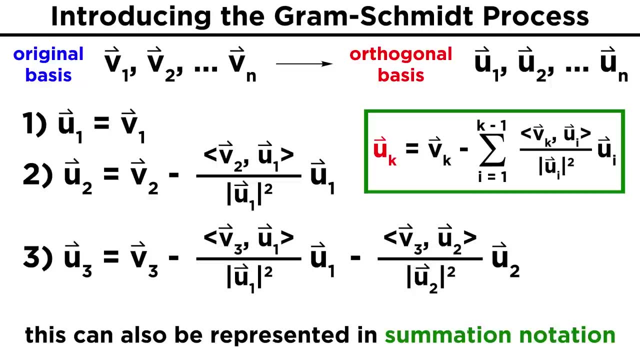 that is not orthogonal to the new vectors we have found, leaving only the orthogonal part. To make things a little more succinct, each of these new vectors, after the first one, can be put into summation notation as follows: U K equals V K minus the sum over I. 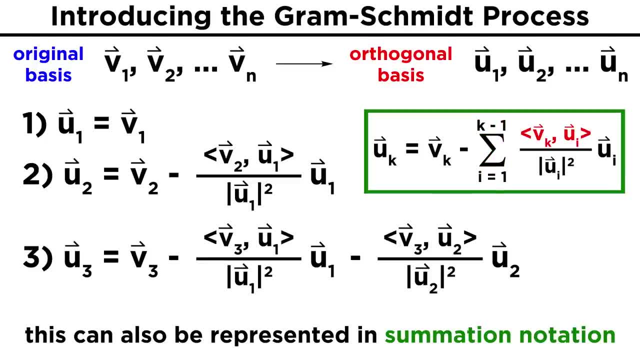 Okay, Okay, Okay Okay. k minus one of the inner product between vk and ui divided by the length of ui, squared times ui. If this notation is unfamiliar, go back and check out some of my tutorials on sums. otherwise we can quickly see how the orthogonal basis we just wrote can be derived from this expression. 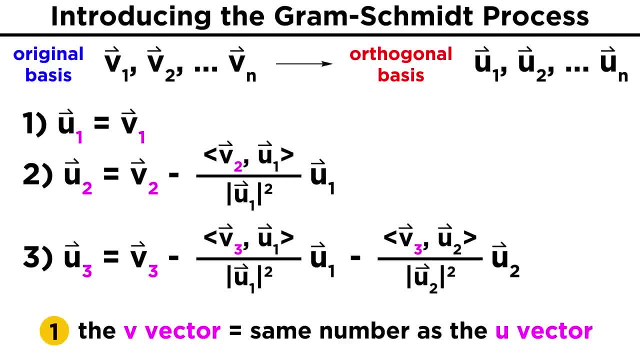 Some useful tips to help remember how this looks include noting that the only v-vector that appears in the formula has the same number as the u that is being found. Also, every other u-vector that has already been found will show up in a specific term. 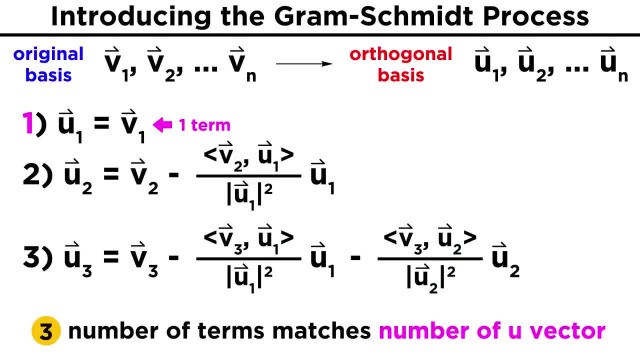 in the remaining v-vectors. Another helpful feature is that u1 has one term in its formula, u2 has two, u3 has two, u3 has three, and so on. For ordinary real vectors, what we mean by inner product is simply the vector dot product. 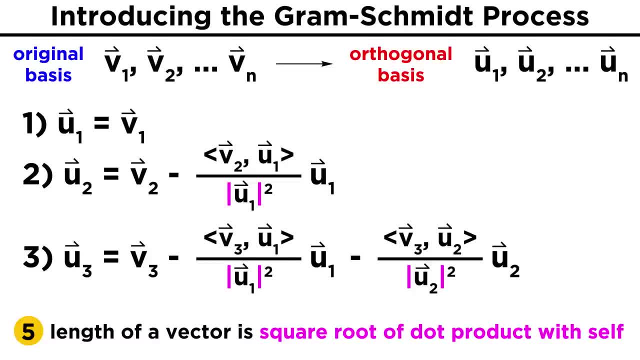 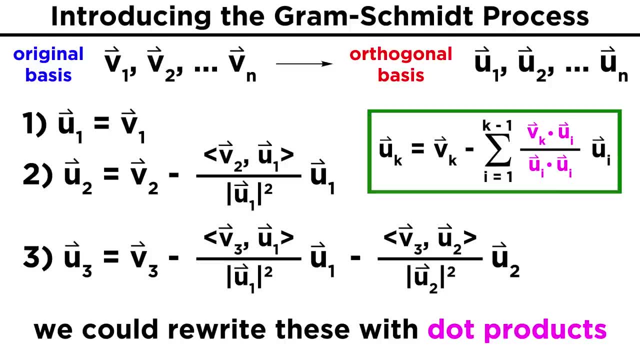 And recall that the length of a vector is simply the square root of its dot product with itself. So just considering this case, we can rewrite these terms with dot products. This might all look a bit overwhelming at first glance, but let's look at an example. 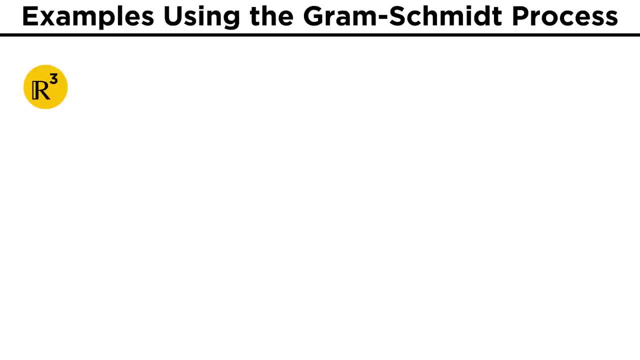 and take it step by step. Consider the basis vectors for R3,: v1 equals one negative one one. v2 equals one zero one and v3 equals one one two. We always start by setting our first vector, u1, equal to the first basis vector, so u1. 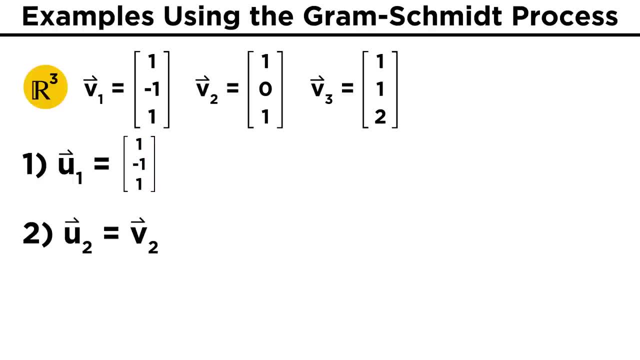 equals one negative one one. Now we get to step two, where we take our second vector, v2, and subtract v2 dot v3.. Well, v2 dot u1 will be one times one plus zero times negative one plus one times one. 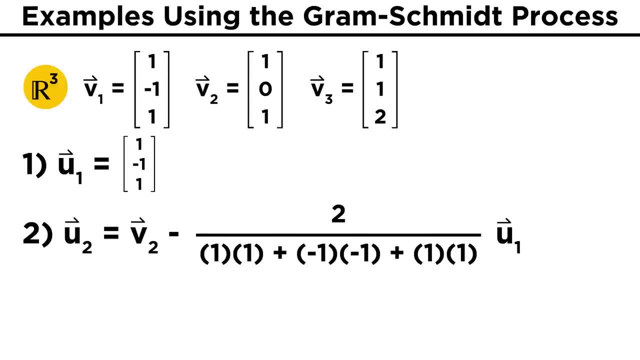 or simply two. Then u1 dot, u1 will be one times one plus negative, one times negative, one plus one times one or three. So u2 equals one zero, one minus two thirds times one negative one plus one times one. Simplifying this expression we get U2 equals one third, two thirds one third. 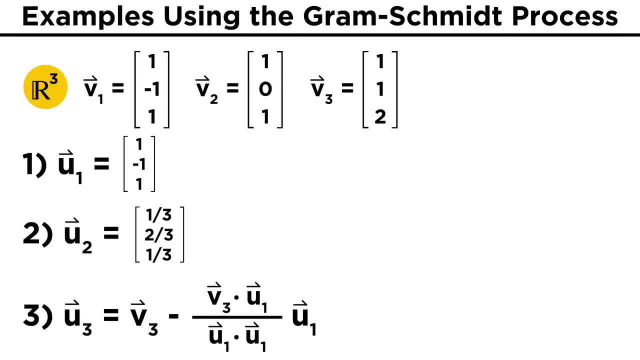 Finally, for the third vector, U3, we will take V3 minus V3 dot U1 over U1 dot U1 times U1, minus V3 dot U2 over U2 dot U2 times U2.. Now, simplifying V3 dot U1 is one times one plus one times negative, one plus two times. 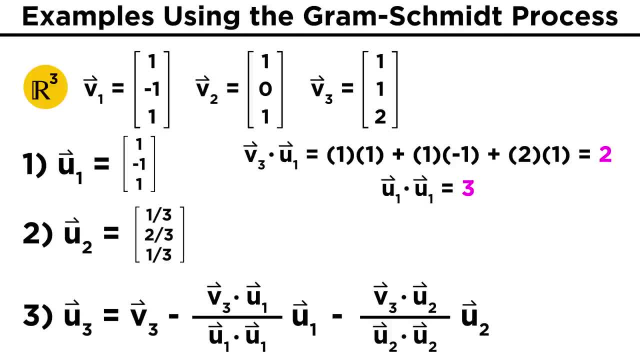 one, which is two. We already know that U1 dot U1 is three, so let's just use that. Then V3 dot U2 is one times one third plus one times two thirds plus two times one third, which equals five thirds. 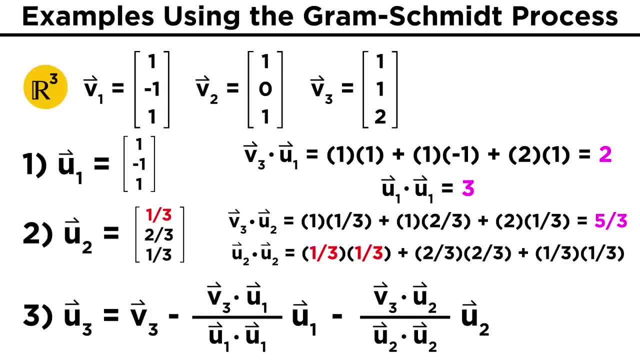 And then U2 dot. U2 is one third times one third plus two thirds times two thirds plus one third. This is one third times one third, which becomes one ninth plus four ninths plus one ninth. This is six ninths, which simplifies to two thirds. 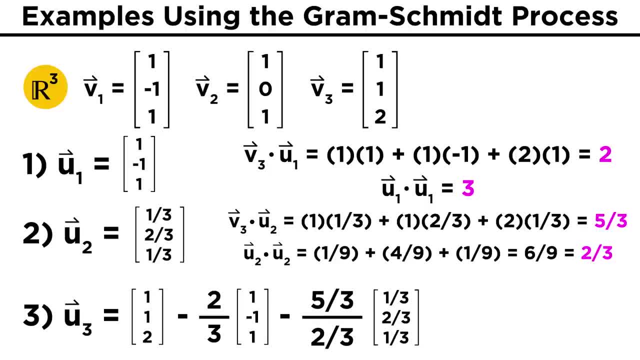 Plugging in all these dot products we get. U3 equals one one two minus two thirds times one negative one. one minus five thirds over two thirds, which simplifies to five halves times one third, two thirds, one third. 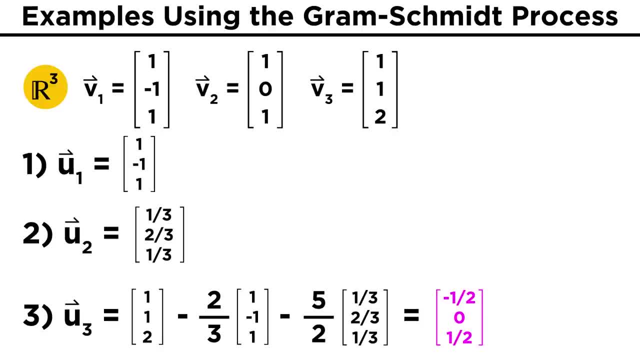 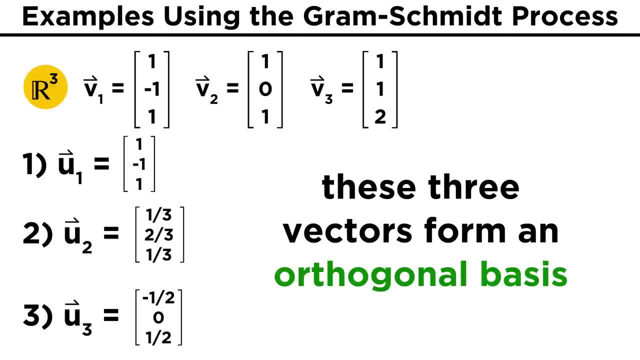 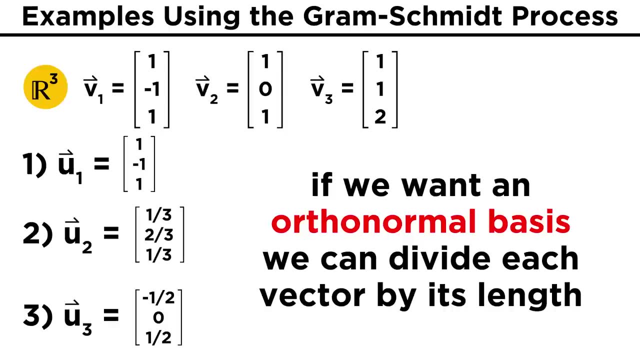 Lastly, going through the vector addition, we end up with: U3 equals negative one half, zero one half. These three vectors form an orthogonal basis. Now, if we wanted an orthonormal basis, as we know, we would take each of these resultant 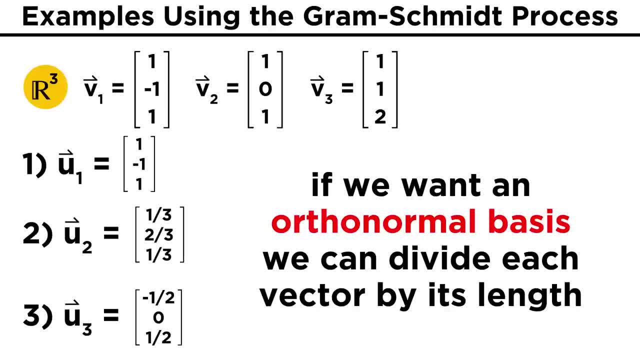 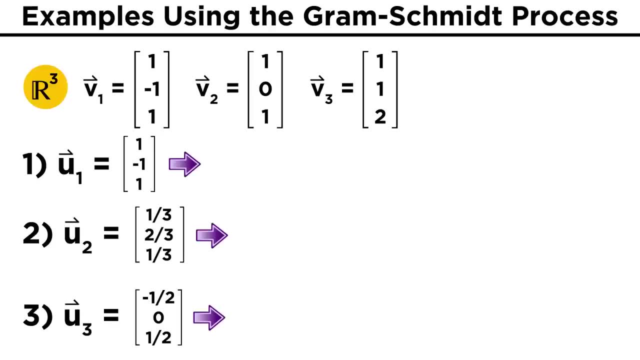 vectors and do what we have already learned: dividing each vector by its length, thus creating a new set of vectors of length one, and since they are already orthogonal, these vectors will be orthonormal. To be thorough, let's go ahead and do this for the three vectors we just found. 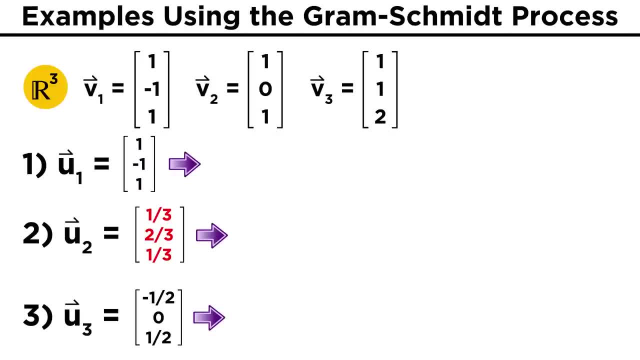 U1 equals one negative one, one, U2 equals one third, two thirds, one third, and U3 equals negative one half, zero, one half. We know that U1 dot U1 equals three, so the length of U1 is root three. 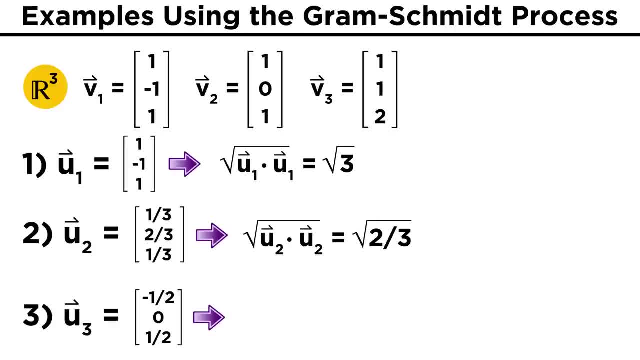 We also saw that U2 dot U2 was two thirds, so the length of U2 is root two thirds. We must still calculate U3 dot U3, which ends up being negative. one half times negative, one half plus zero times zero, plus one half times one half, which equals one half. so 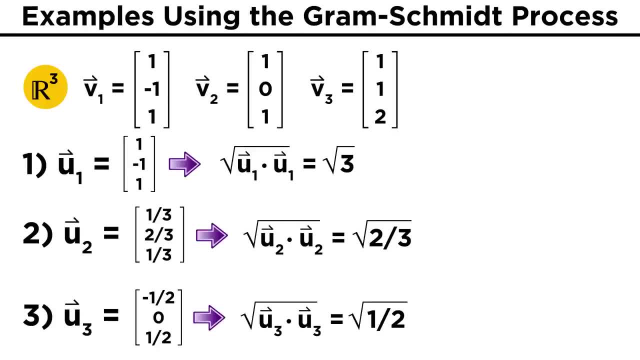 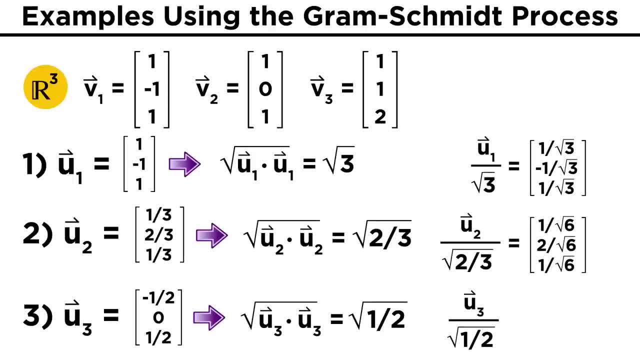 Two over root six. one over root six. Finally, dividing U3 by its length, we get negative root two over two, zero root two over two. These are the orthonormal basis vectors we obtain from our original basis thanks to. 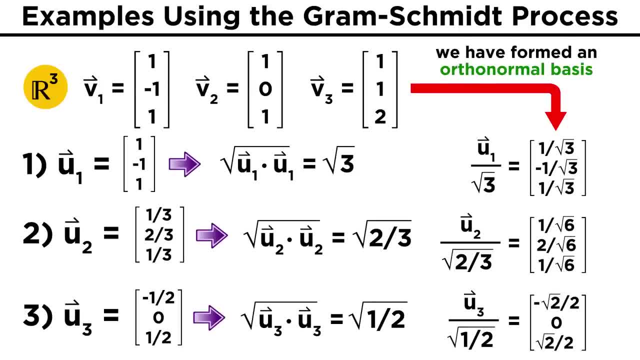 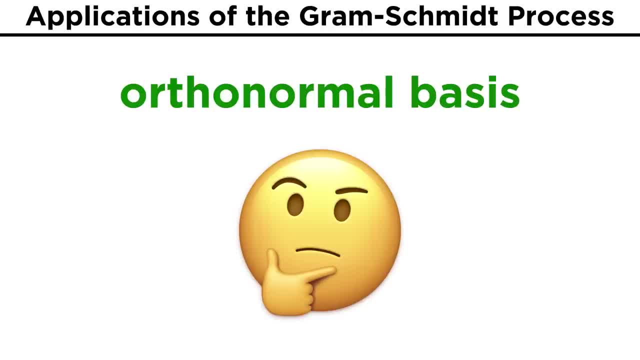 the Gram-Schmidt process. Being able to generate an orthonormal basis is a useful tool, as the bases themselves can very helpful for certain calculations. This process also works for different kinds of vector spaces, such as ones involving functions. it just changes how we compute the inner product.